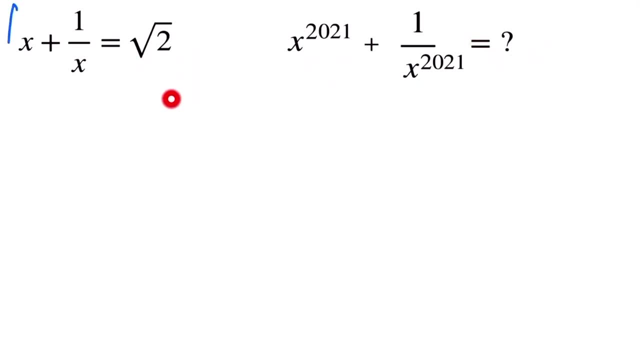 the value of this. So for finding the value of this at first, we notice in this part of the question, x plus 1 by x is equal to under root 2.. So now we square it on both side, So like that. So now we break this on the identity, a plus b, the whole square. a square plus b square. 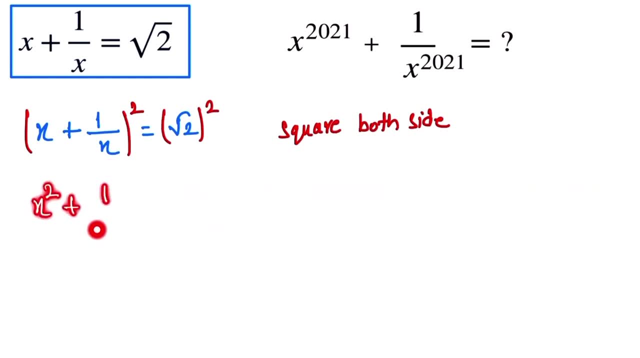 plus 2ab. So this one is x square plus 1 by x square, plus 2 into x, into 1 by x is equal to 2.. Now this one is cancelled. So here is: x square plus 1 by x square is equal to 0, because this one. 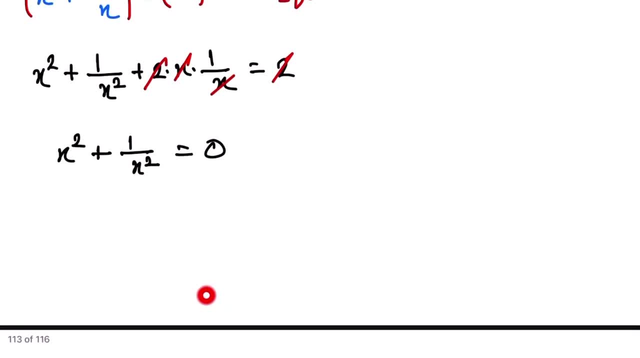 2 and 2 is cancelled. So now we take the LCM, So here is x square and here is x to the power 4 plus 1.. We add the power, So here is x to the power, 4 plus 1 and it becomes 0.. So the value. 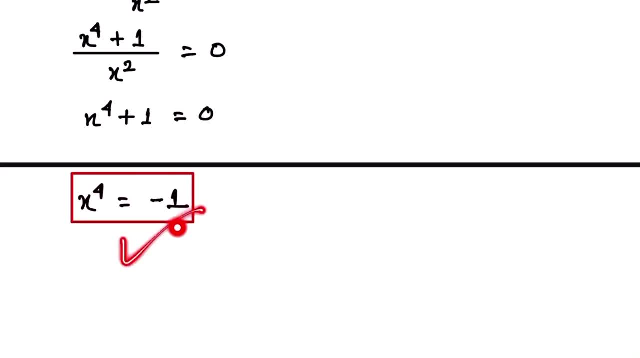 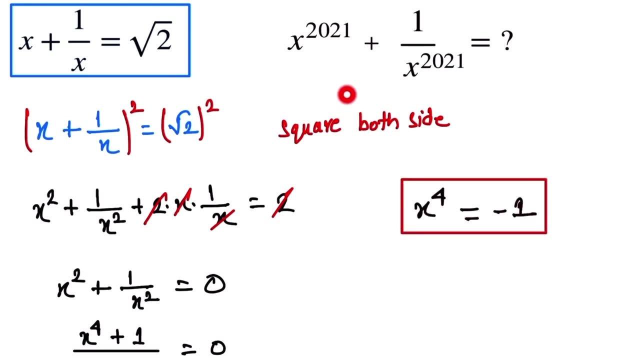 of x to the power 4 is equal to minus 1.. Here we got the value of x to the power 4.. x to the power 4 is equal to minus 1.. So now we notice in this part of the question, x to the power 2021 plus 1 by x to the power 2021.. So here, 2020. 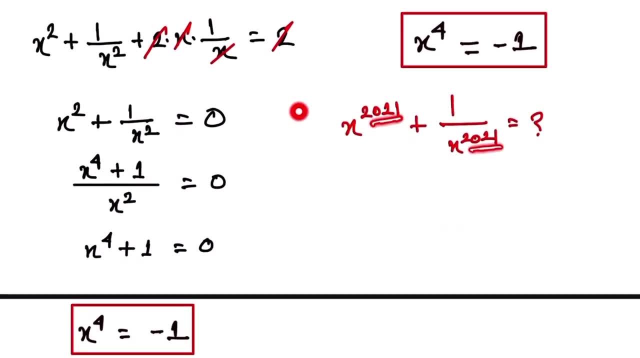 2020 can be written as 4 into 505.. So now we break this. So here is x to the power 4.. The whole power is 505 into x, plus 1 by x to the power 4.. The whole power is 505 into x. So now we put the value of 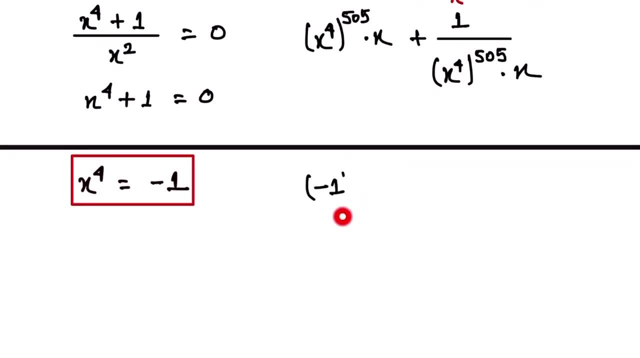 x to the power, 4 minus 1.. So it is minus 1.. The whole power is 505 plus into x, plus 1 by minus 1.. The whole power is 505 into x. So here this one is the odd number. So when 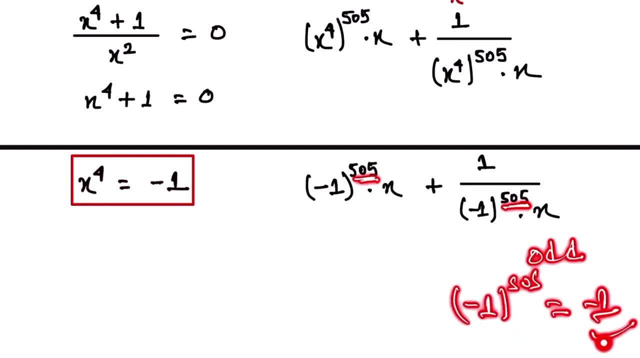 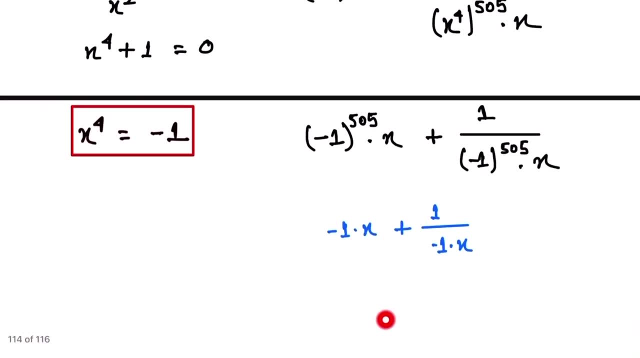 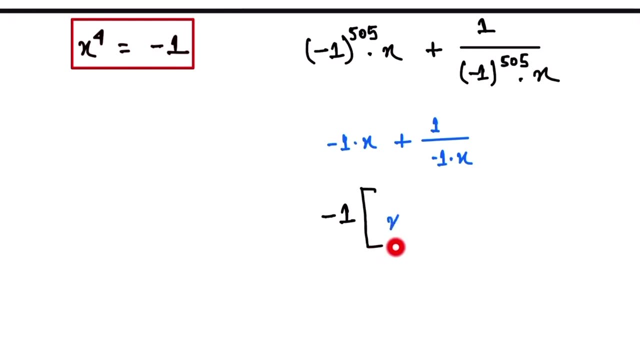 we power the 1 by odd number, It gives the same value. So here is minus 1.. So minus 1 into x, plus 1 by minus 1 into x. So now we take the minus 1 as a common. So here minus 1 into x, plus 1 by x. So now: